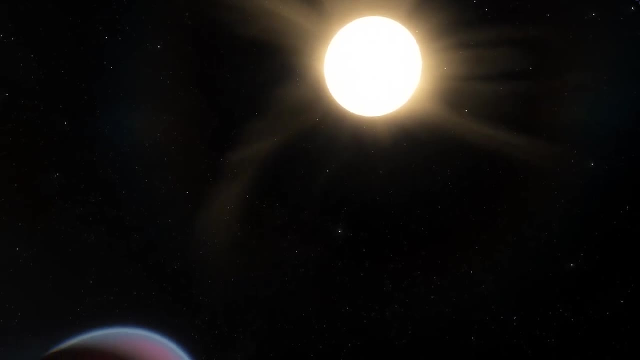 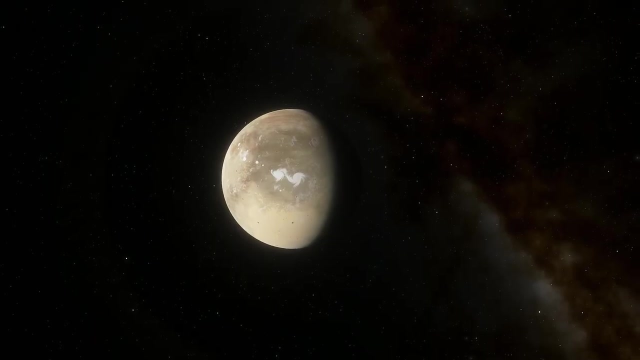 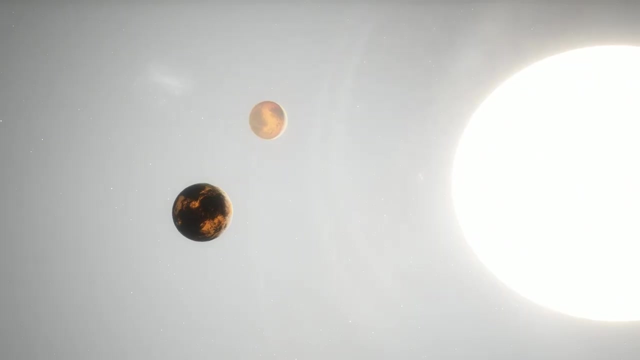 of our solar system. Pegasi b, aka Dimidium, was a groundbreaking find that confirmed planets like Earth could exist elsewhere in the universe. As of 1 October 2019, there are 4,118 confirmed exoplanets in 3,063 systems, with 669 systems. 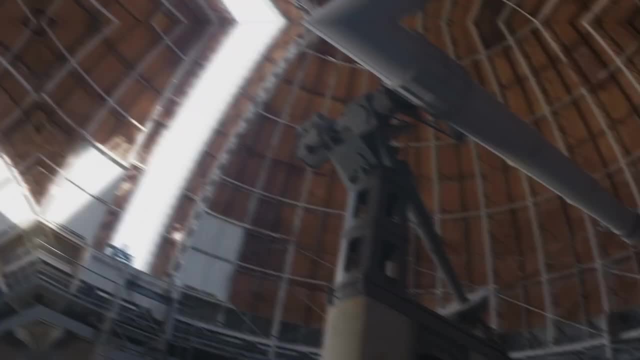 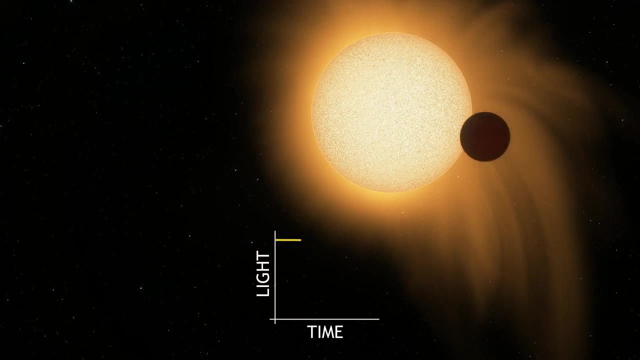 having more than one planet. There are many methods for detecting exoplanets. For example, transit photometry is a phenomenon when a celestial body, in this case a planet, passes directly between its host star and the observer As viewed from a particular 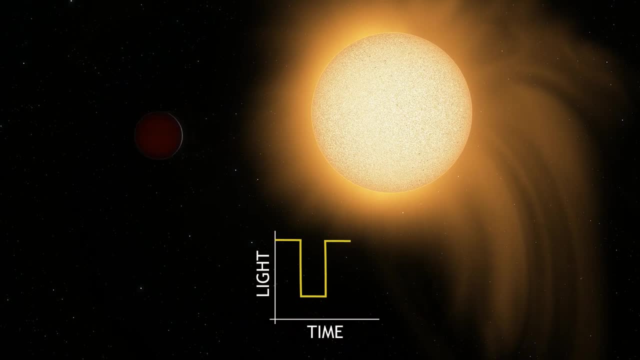 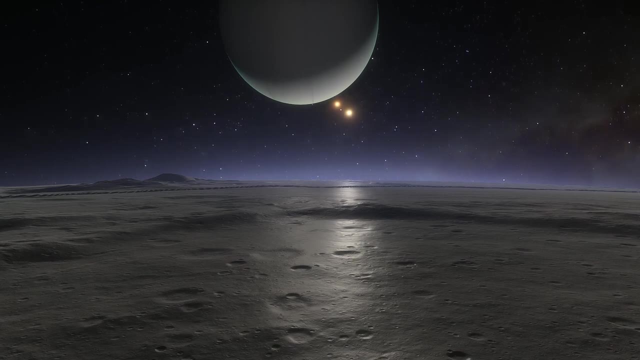 vantage point, the transiting planet appears to move across the face of its parent star, covering a small portion of it. Doppler spectroscopy is another common method used to indirectly discover exoplanets. It is also known as the wobble method because 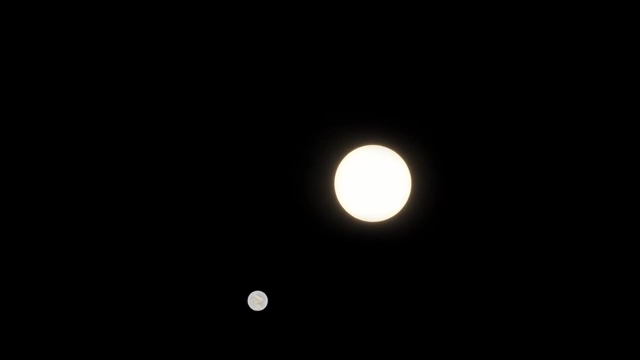 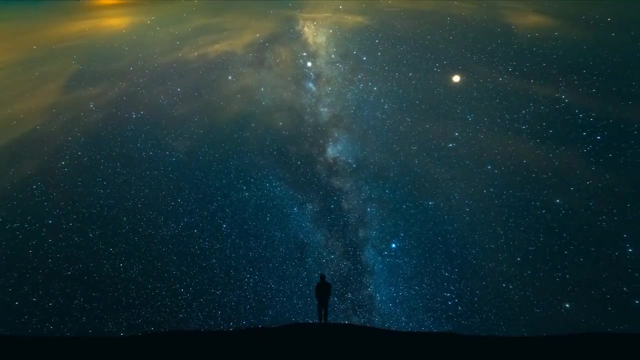 the planet's gravity affects the star's motion, and both the planet and its parent star orbit a common centre of mass. But we can't see the movement of the stars because they are very far away from Earth. Instead, astronomers use the Doppler effect. when a 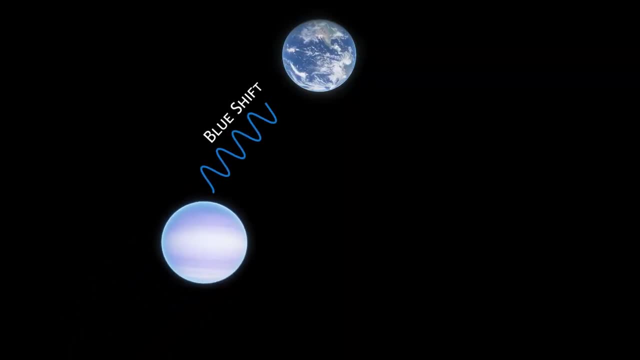 planet moves towards us, It has a higher light frequency, or a blue shift, and when it's moving away from us, its red shifts a lower light frequency. Both the transit and the wobble method have found the most exoplanets, but these methods 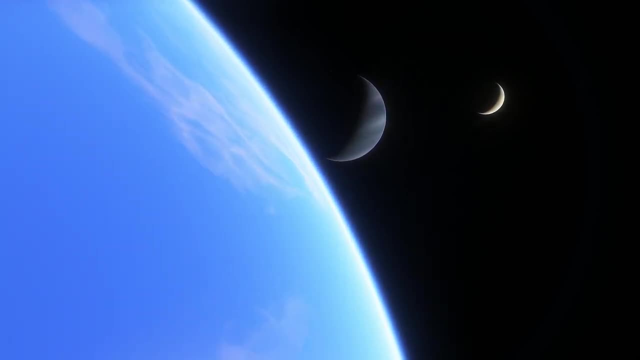 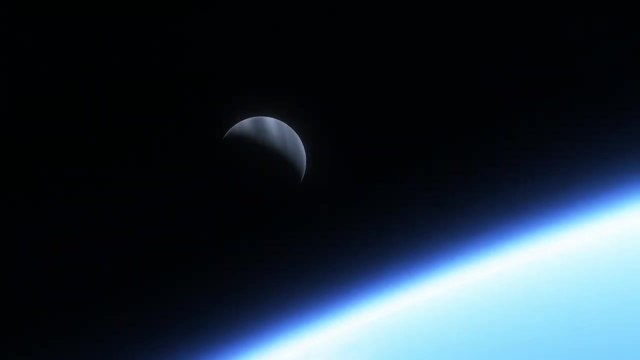 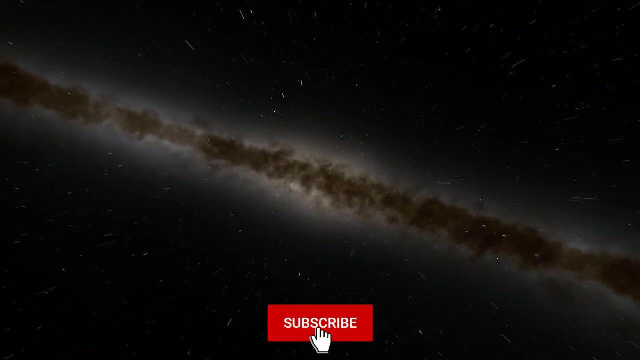 suffer from a clear observational bias favouring the detection of planets near the star. Thus, 85% of exoplanets detected are inside of planets. So far, almost all of the exoplanets detected are within the Milky Way: About 1 in 5 sun-like. 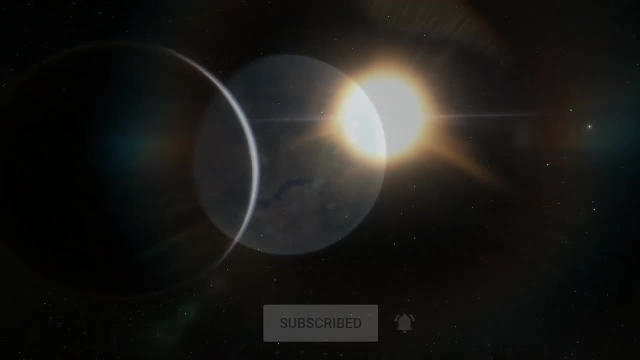 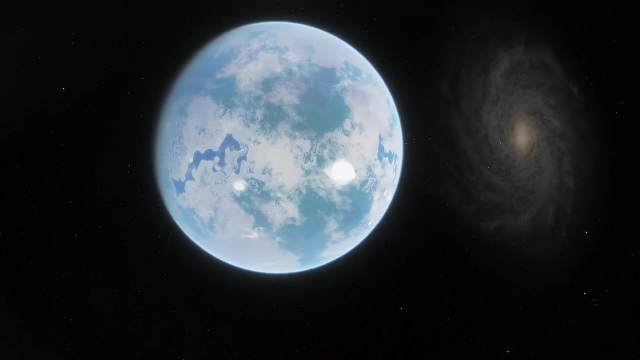 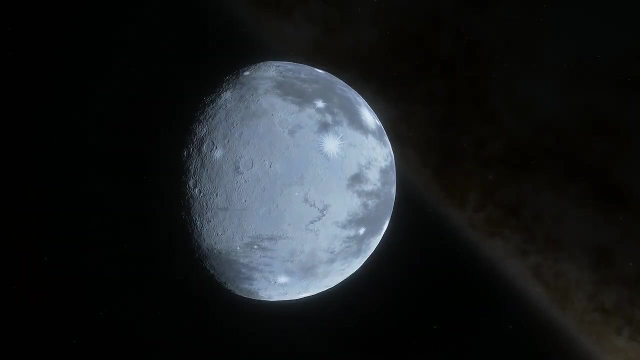 stars have an Earth-sized planet in the habitable zone. Assuming there are 200 billion stars in our galaxy, it can be hypothesised that there are 11 billion potentially habitable Earth-sized planets in the Milky Way alone. The least massive planet in the Milky Way is the Milky Way. The Milky Way is the largest. 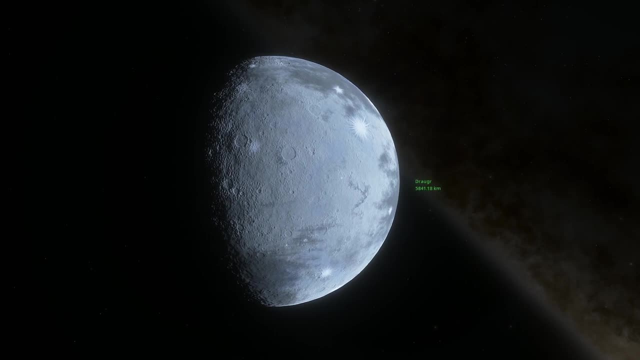 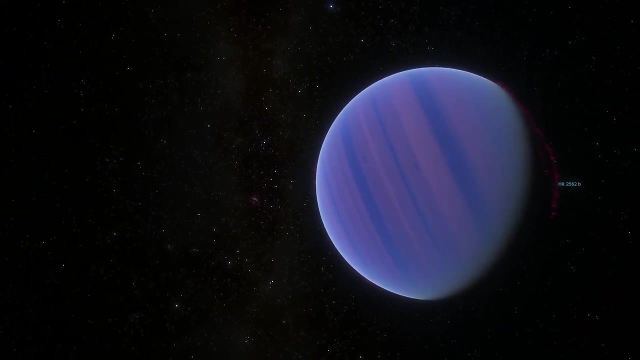 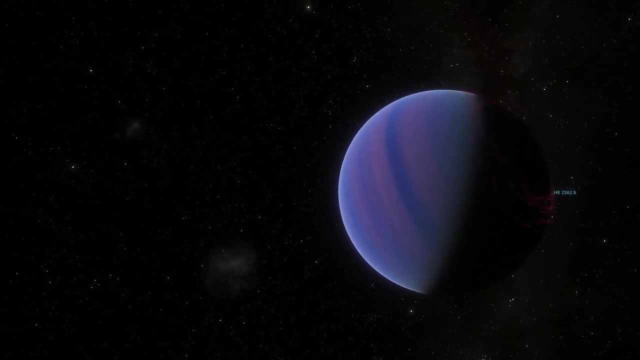 planet known is Dragoor, which is about twice the mass of our Moon. The most massive planet listed on the NASA Exoplanet Archive is HR2562b, about 30 times the mass of Jupiter, although according to some definitions of a planet, it's too massive to be a planet and may be. 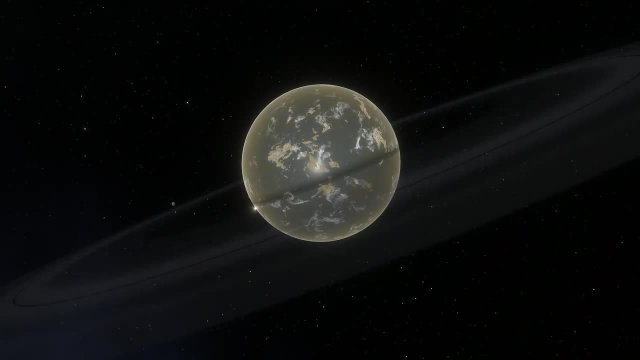 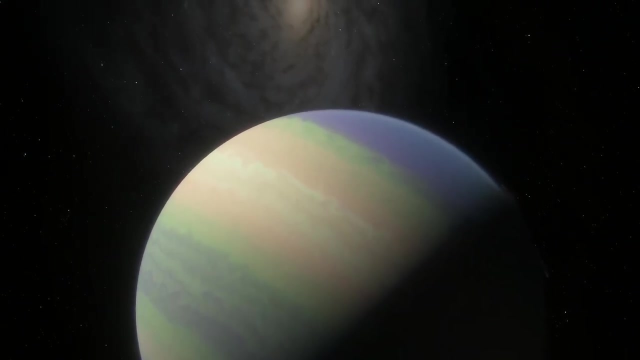 considered a brown dwarf instead. Besides exoplanets, there are also rogue planets which do not orbit any star. These tend to be considered as a separate category, especially if they are gas giants, in which case they are often counted as sub-brown dwarfs. Rogue- 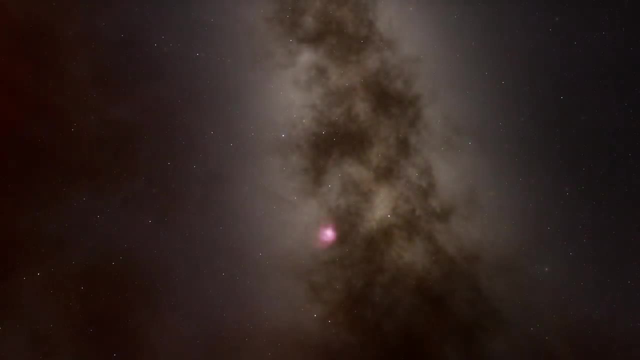 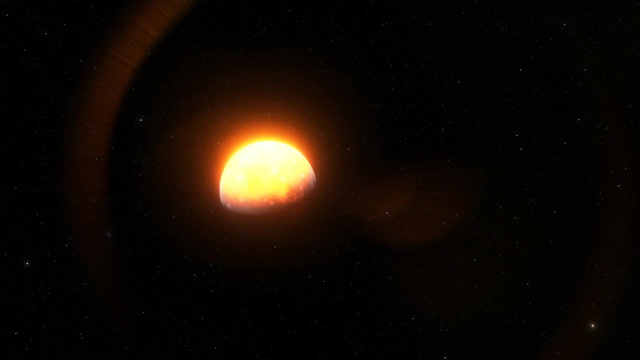 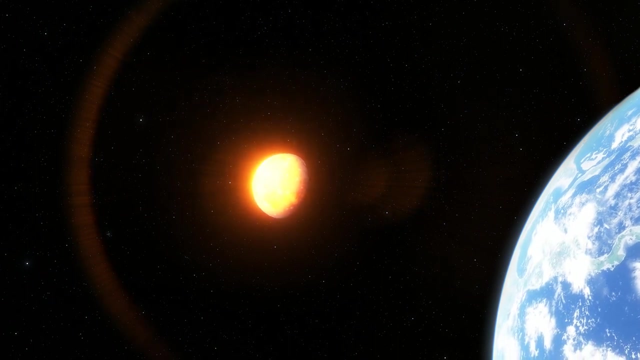 planets in the Milky Way possibly number in the billions or more. That's why some people paid special attention to the Nibiru Cataclysm, which is a supposed disastrous encounter between Earth and a large rogue planet, sometimes referred to as Nibiru or Planet X. Fortunately, 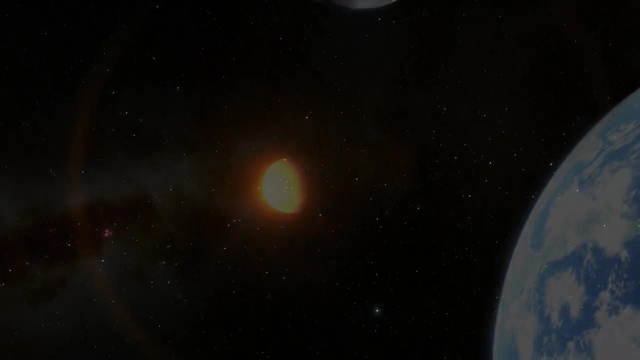 there is no evidence of such an object heading our way. In 2004,, an exoplanet with a mass of 8.6 million stars was discovered. An exoplanet with a mass of 8.6 million stars is considered a super-Earth planet, with a mass of 8.6 times that of Earth. 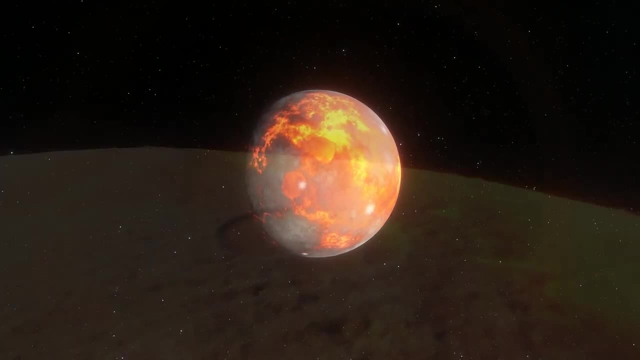 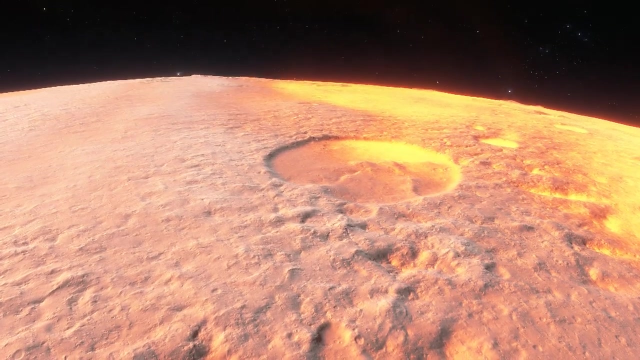 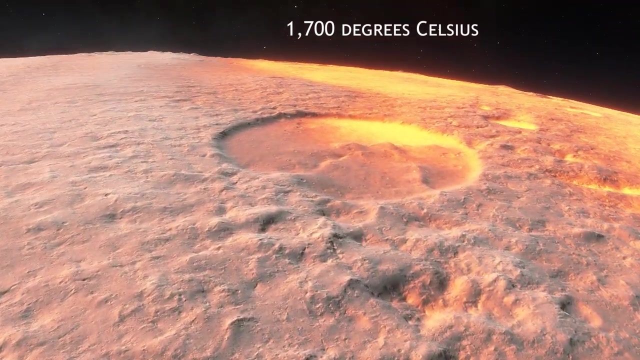 Spawning a class of exoplanets known as super-Earths. 55. Kenseri E is a volcanic hellish world located 41 light-years away from us. The side of the planet facing its star has temperatures more than 1,700 degrees Celsius. Large surface temperature variations on Kenseri have been 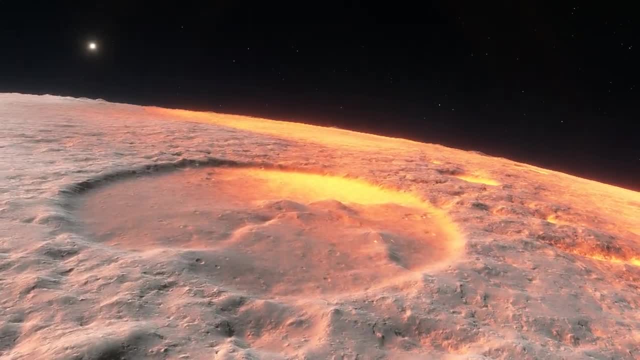 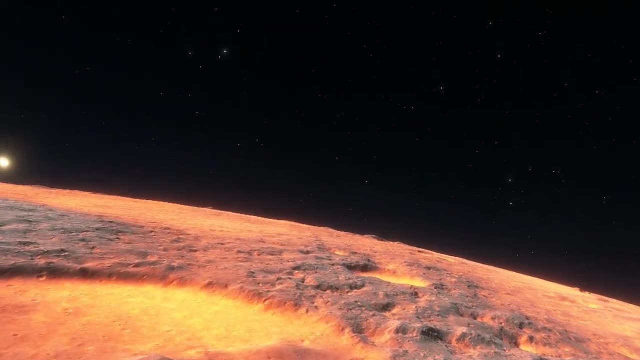 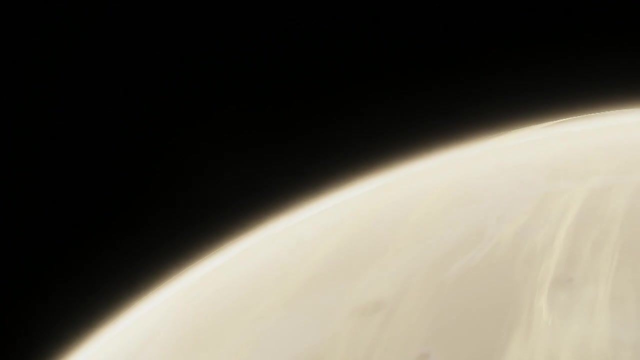 attributed to possible volcanic activity releasing large clouds of dust which blanket the planet and block thermal emissions. The discovery of exoplanets has intensified interest in the search for extraterrestrial life. There is special interest in planets that orbit in a star's habitable zone, where 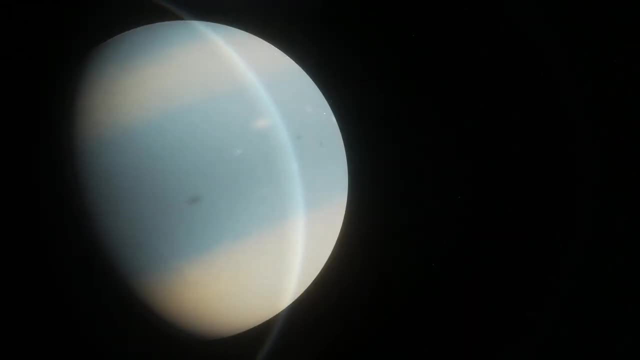 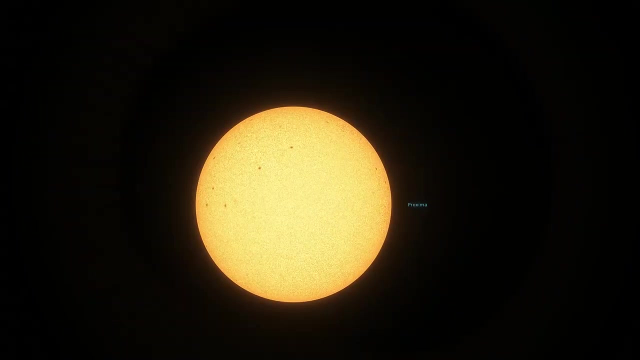 it is possible for liquid water. The nearest exoplanet is Proxima Centauri b, located 4.2 light-years from Earth and orbiting Proxima Centauri, the closest star to the Sun. So it takes light the fastest thing there is in the universe to get to the Earth. Proxima.